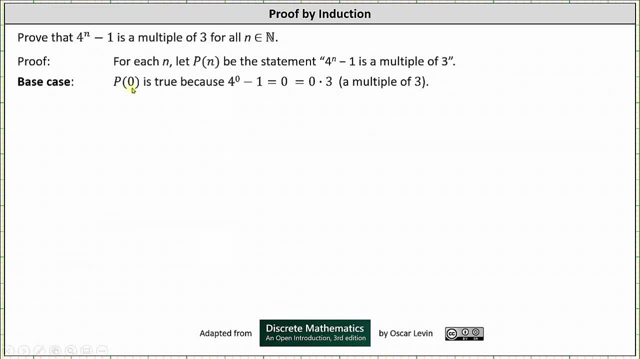 If your text doesn't include zero as a natural number, you would consider p of one. P of zero was true, because four to the power of zero minus one is one minus one, which is zero, and zero times three is zero, showing that zero is a multiple of three. 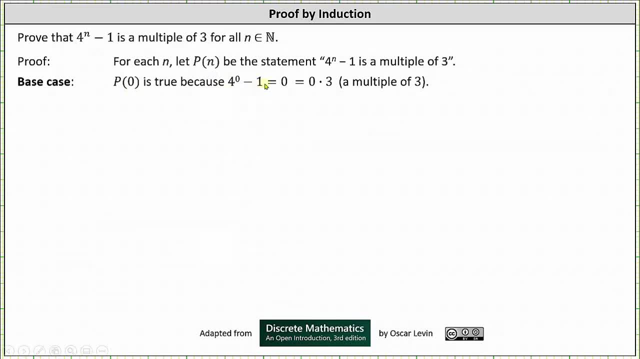 Notice, p of one would be four to the power of one minus one, which is three. and of course three is also a multiple of three. And now we consider the inductive case, where we let k be a natural number and we assume p of k is true. 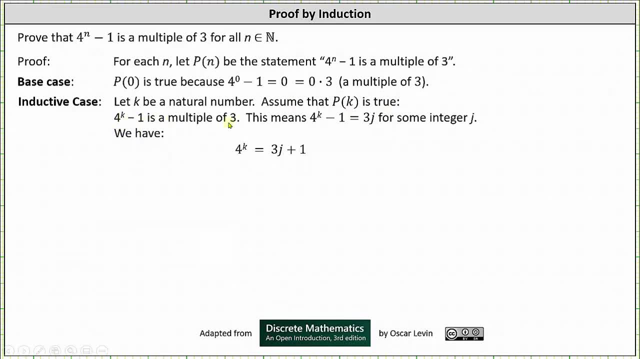 which means four to the power of n minus one is a multiple of three. Well, if four to the power of k minus one is a multiple of three, then four to the power of k minus one must equal three times j, where j is some integer. 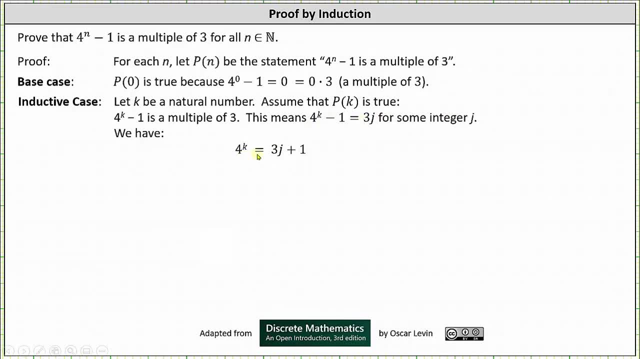 From here, if we add one to both sides of the equation, we have four to the power of k equals three j plus one. And now we need to show that p of the quantity k plus one is true, meaning four to the power of k plus one. 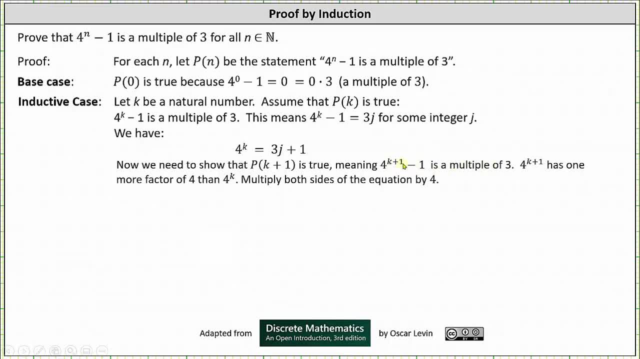 minus one is a multiple of three. Four to the power of k plus one has one more factor of four than four to the power of k. Our next step is to multiply both sides of the equation by four. Multiplying on the left side of the equation. 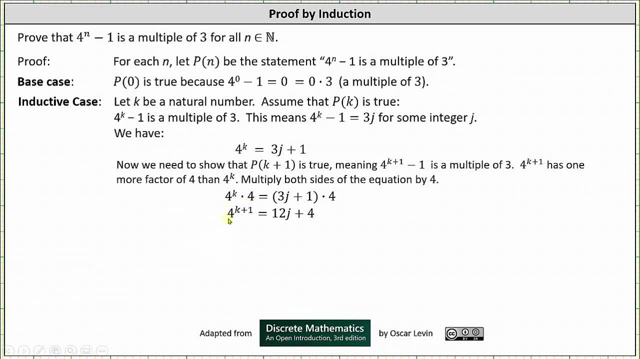 four to the power of k times four is equal to four to the power of k plus one. On the right side of the equation, distributing four, we have 12j plus four. And now we need to write the left side of the equation. 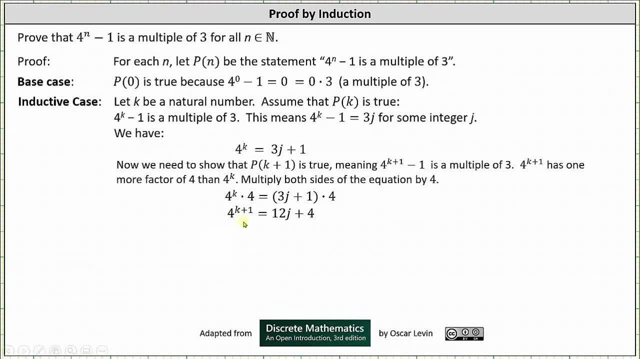 in the form of four to the power of k plus one minus one, which means our next step is to subtract one from both sides of the equation. This gives us four to the power of k plus one minus one equals 12j plus three. 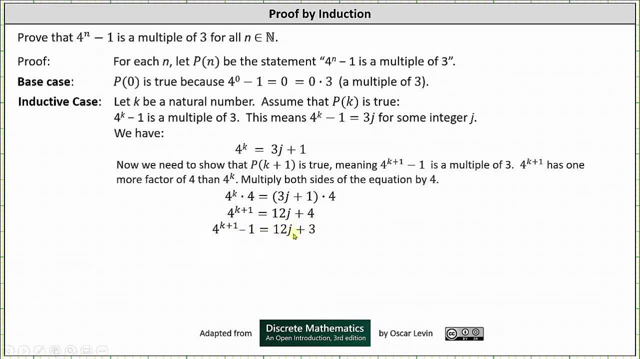 And now notice the right side of the equation has a common factor of three. We can write the right side of the equation as three times the quantity four j plus one, And since four to the power of k plus one minus one is equal to three times the quantity four j plus one. 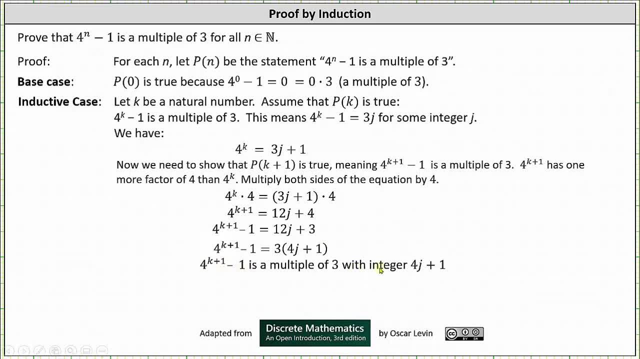 four to the power of k plus one minus one is a multiple of three with the integer of four j plus one. Thus p of the quantity k plus one is true, completing the inductive case. Therefore, by mathematical induction, the statement p of n is true for all natural numbers n. I hope you found this helpful. 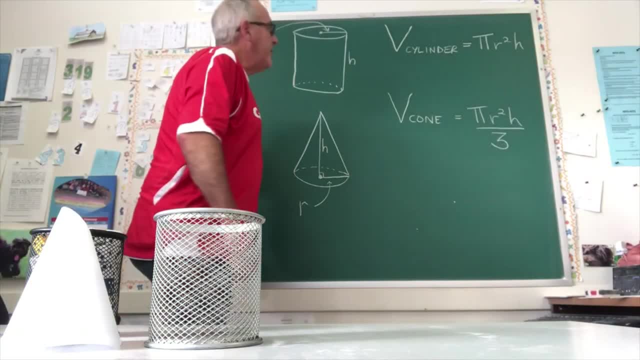 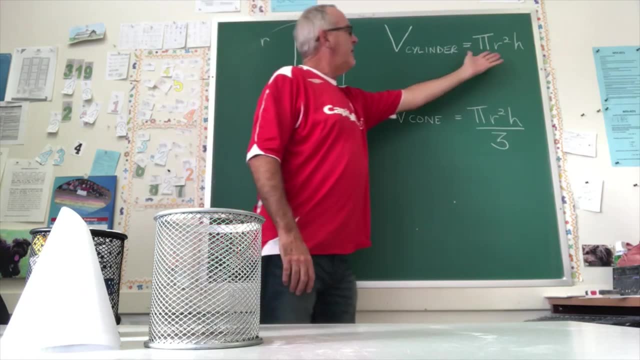 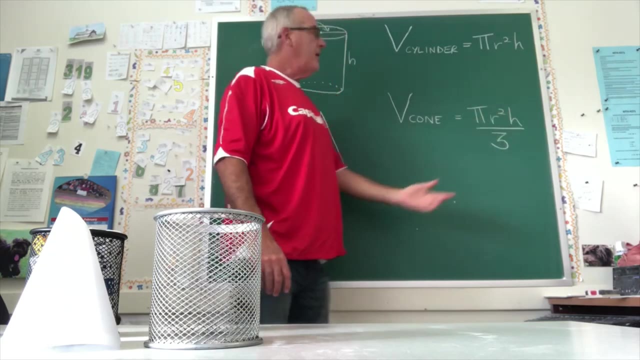 Some students are a little surprised when they start working with the volume of a cylinder formula and the volume of a cone formula and notice that the things in the formula are the same, except for the cone. we're dividing by three. Here I have a diagram of a cylinder and a diagram of a cone. Both 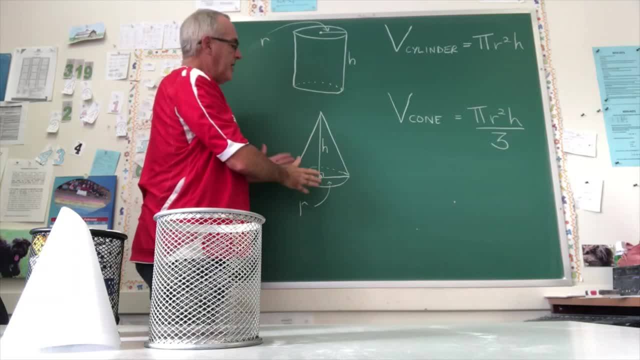 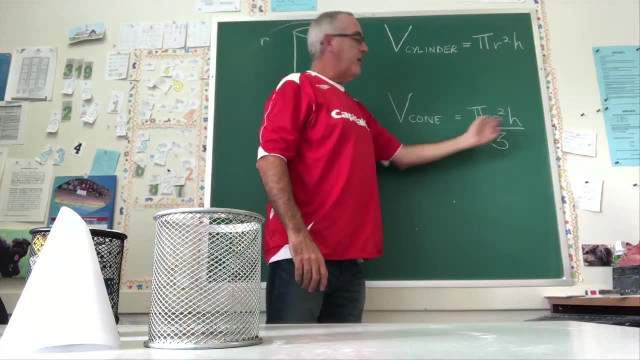 diagrams show the radius and the height and I chose to make them have the same height and the same radius. Notice that Pi r squared is part of both formulas. Pi r squared, of course, is the area of a circle formula. The cylinder has a circle. 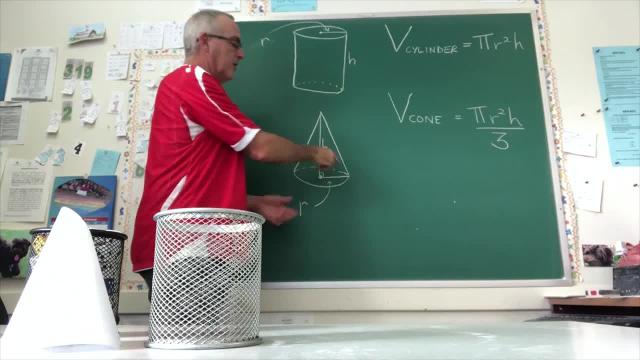 at the bottom end, at the top, and that cone has a circle at the bottom. if you have it opening downwards, What we do is we take the area of that circle and we multiply it by the height in order to get our volume, but again, the volume is always constant. This means that we have various factors, including how much we can only connect or connect to η in our stump. 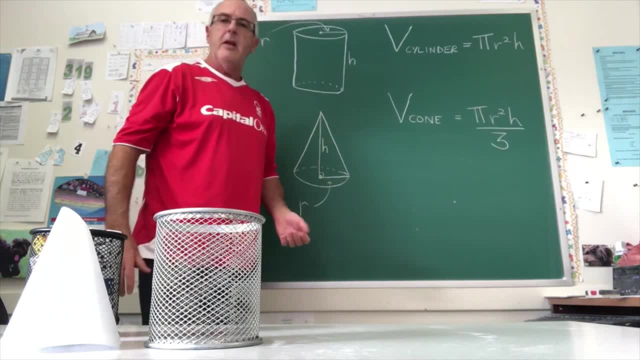 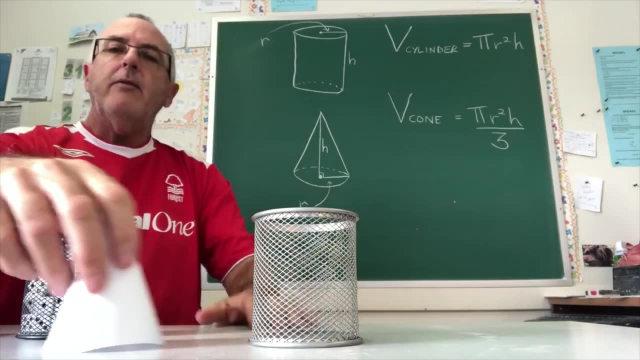 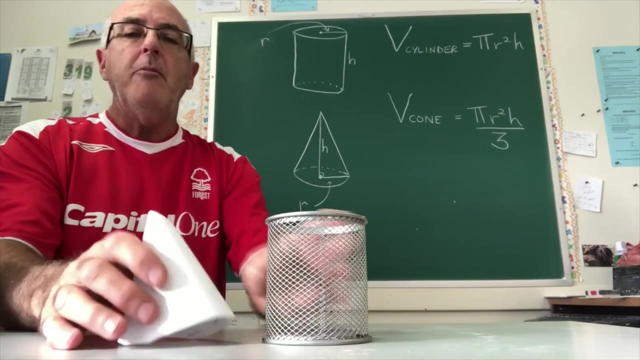 volume of the cone. all of that's divided by three. So let's illustrate what that looks like. Here I have a cylinder and I have a cone which has the same height as the cylinder. They also have the same radius. I'm going to fill this cone with these dice. Dice are not the best. 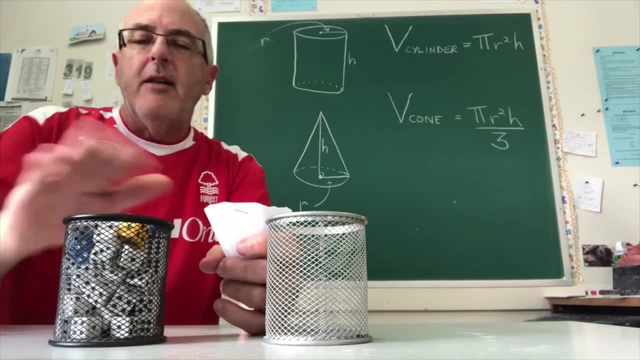 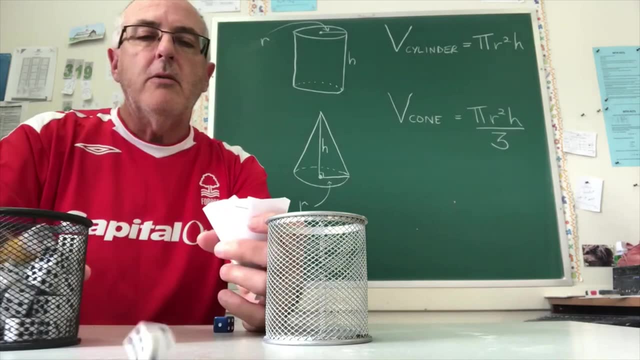 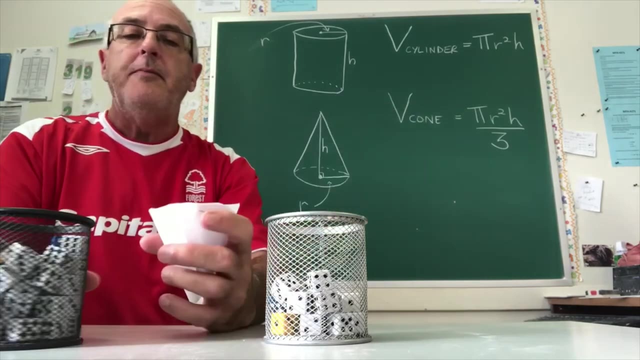 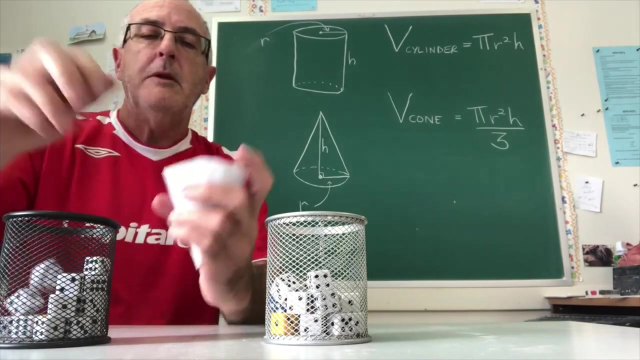 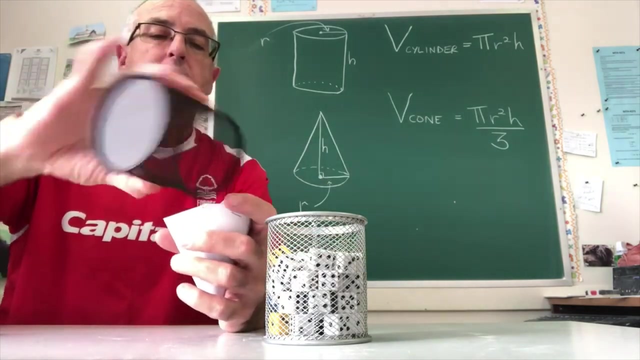 thing to use to measure volume, because they are. there are spaces in between them, but it's good enough for us to illustrate this idea. So I fill the cone and then I pour it into the cylinder, and then I do it again, Pour it into the cylinder, and finally I'm doing it one last time. So three times I have filled this. 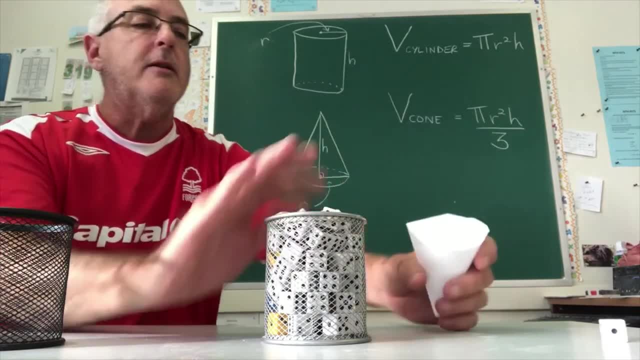 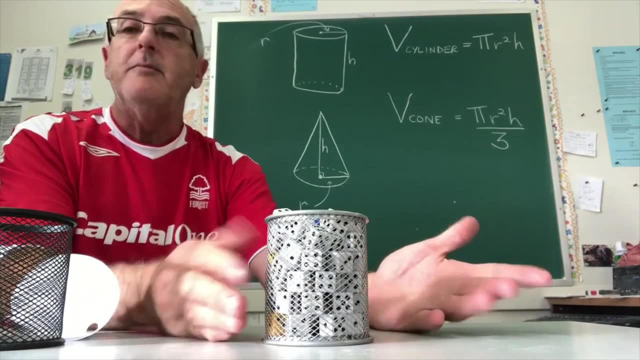 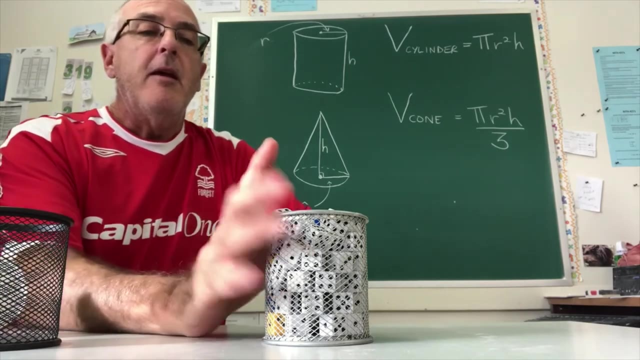 cone with the dice And pour it into the cylinder and, with the exception of one escaping dice, what we can see is that the cylinder is full. So it's true. So long as the cone and the cylinder have the same height and the same radius, the volume of the cylinder will be exactly three times the volume.